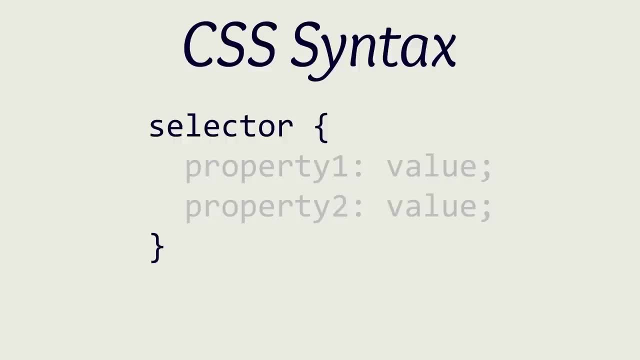 Everything in between these curly brackets will be styles that are applied to the HTML elements that match the selector. Lastly, inside the curly brackets is one or more property-value pairs. Each of these pairs defines a property such as color, font, size, width, etc. and a value for that property. 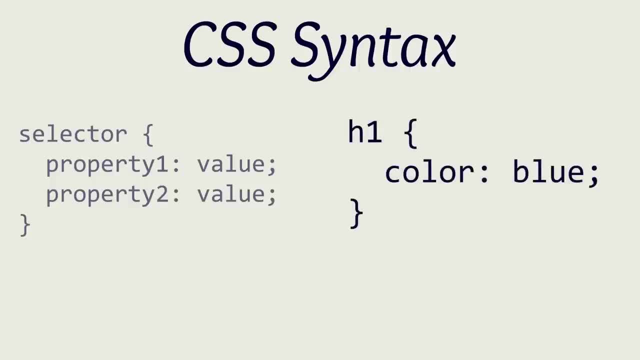 A basic example of the CSS syntax will be setting the text color of all H1 elements to blue. Now that we have the syntax out of the way, let's focus on the various selectors. CSS contains many different types of selectors, but the main selectors are element, class and ID selectors. 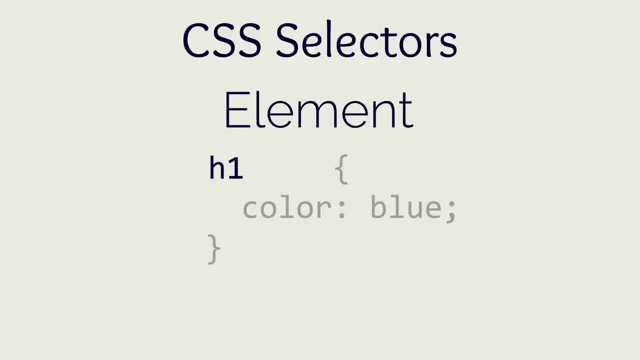 We've already seen the element selector in the previous example of turning all H1s blue. Any HTML element can be used as a selector and the style that is defined for that selector will apply to all HTML elements of that type. By far the most common and useful selector is the class selector. 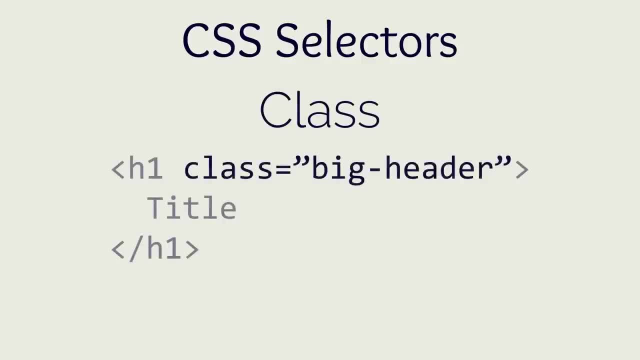 The class selector lets you select HTML elements based on their class attribute. If you remember from my HTML series, all HTML elements can have attributes assigned to them, such as the href for an anchor tag. A class is just an attribute that all HTML elements can have and is used with CSS to distinguish elements for specific styling. 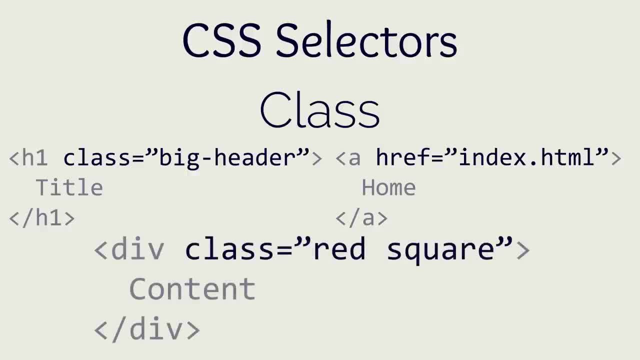 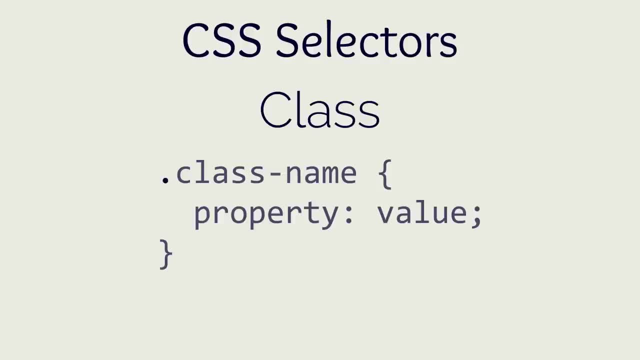 The class attribute can also be used to define a class. It can also have multiple different classes in the same attribute, as long as they're separated by a space. In order to select an element by class, we need to use a period before the class name as the CSS selector. 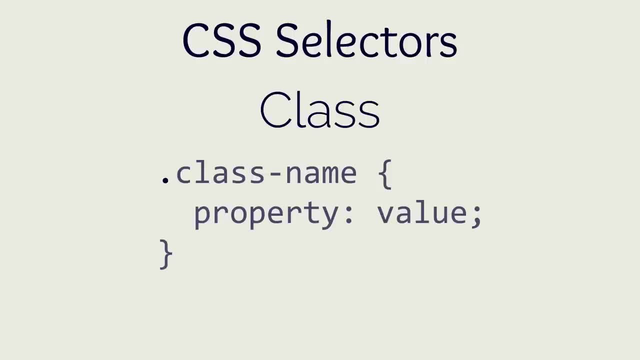 This period tells CSS that whatever follows is a class name and not an HTML element name Classes are the most common selector used because they are amazing for creating reusable components. For example, if you have a site with three different types of buttons that all share the same basic styling but have a different color. 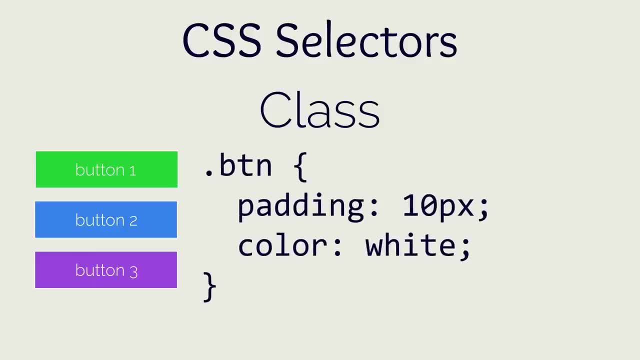 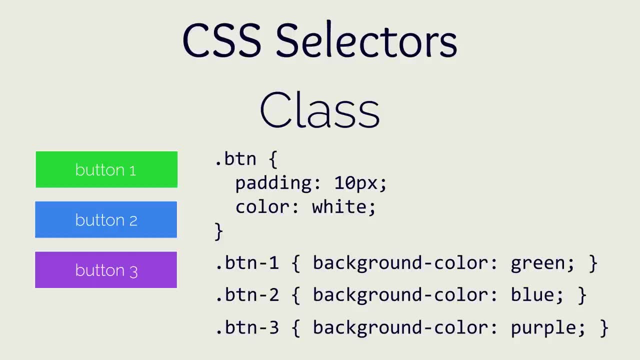 you can use one base class of button to define all of the styles shared between all buttons. You can then have three other classes that define the specific color for the button. Then all you need to do is add both the base button class and your color specific class to your HTML button element. 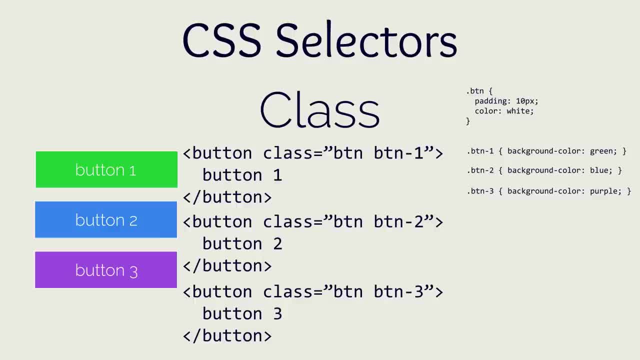 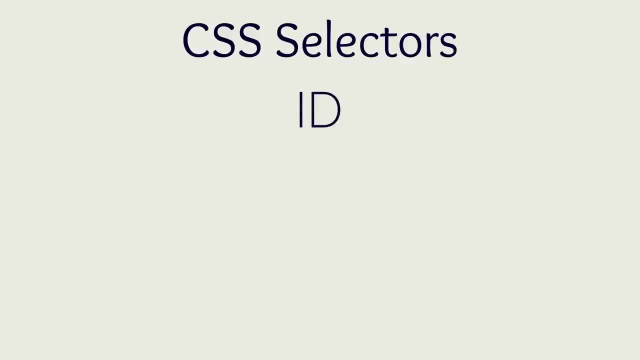 and it'll have all the styles defined in the base button class and the color specific class. The last common selector is the ID selector. The ID selector is very similar to the class selector in that it is an HTML attribute, but an element can only have one ID, while it can have multiple classes. 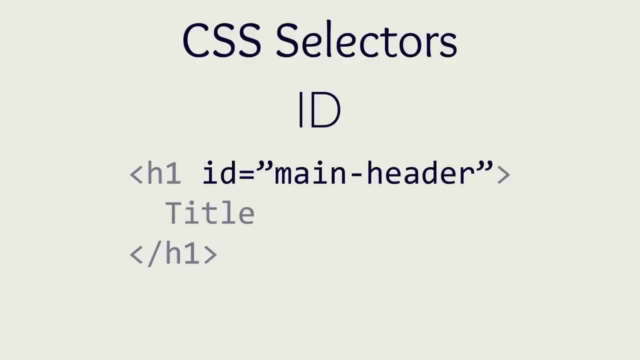 An ID also should be unique across the entire web page, but HTML does not actually enforce this. To use an ID as a selector, you simply need to use a pound sign followed by the ID name, much like how classes use a period followed by the class name. 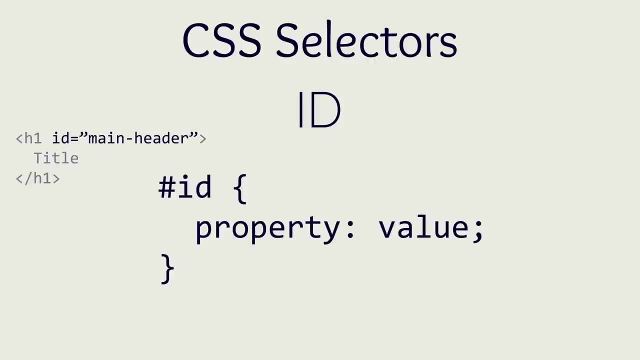 Our previous example is impossible to do with IDs, since IDs are supposed to be unique across the web page and each element can only have one ID. Because of this, I very rarely use IDs. In 99% of all my CSS, I use class selectors and avoid using HTML and ID selectors as much as possible. 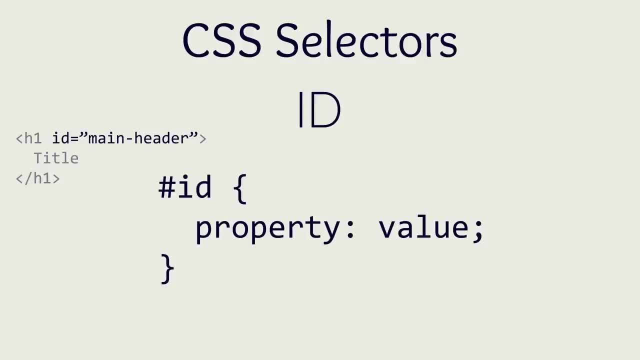 On top of having many different selectors, CSS has multiple different ways to combine selectors together to make your selectors more specific. The first way to combine selectors is to specify multiple selectors that an element must have in order to be styled. To do this, you need to write the various different selectors together. 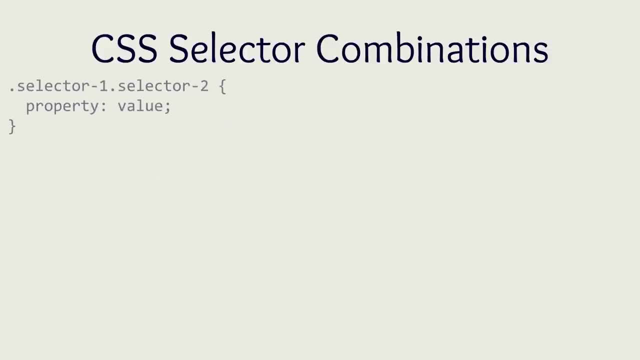 with no spacing between them. For example, if you wanted to select all H1 elements with the class large heading, then you would write the following selector: If you wanted to select an element with the ID big blue and both the class large and blue, 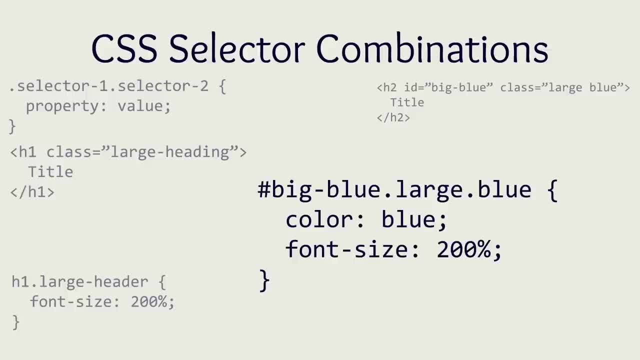 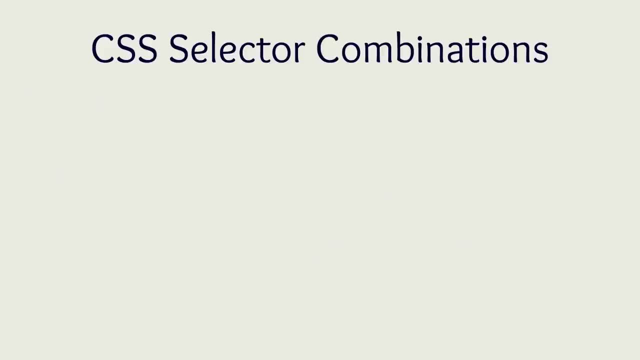 then you would use this selector. All HTML selectors can be combined in this way as many times as you want to create specific or general rules. Another way to combine selectors is to use multiple selectors to specify an ancestor of an element. To do this, you will put a space between the ancestor and child selector. 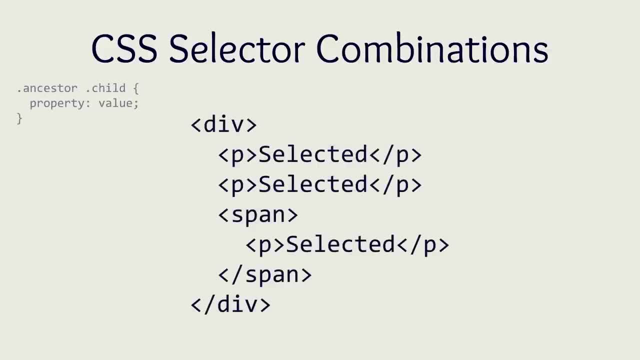 For example, to select all P tags inside a div, you simply need to use the following selector: This will select all P tags that have a div as their ancestor, even if the div tag is not the direct parent of the P tag. This combination of selectors can be combined with the previous combination of selectors. 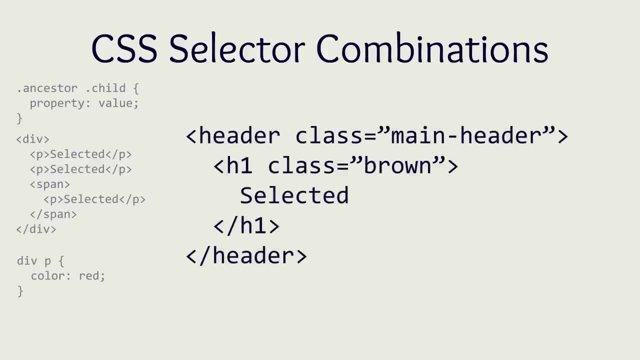 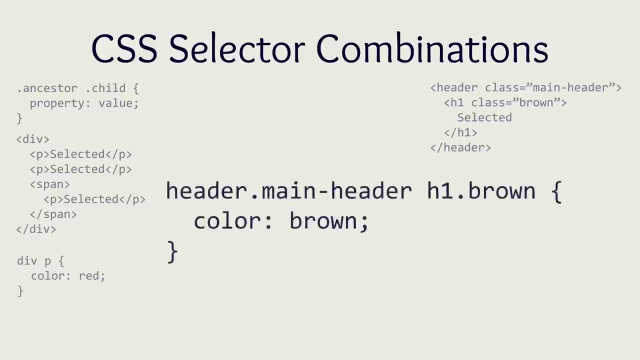 to make even more specific selectors, For example, to select all H1 tags with the class of brown that have a header with the class main header as their ancestor. you would do this. The last common combination of selectors is when you want to share a set of style properties. 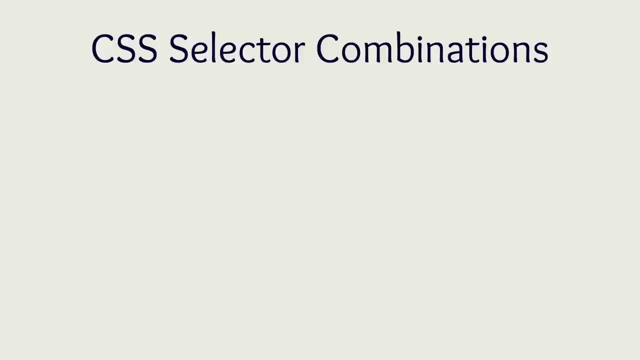 and values between multiple selectors. If you have a class big and another class large that both have the same style, properties and values, then you can combine these selectors into one selector by using a comma between the selectors. This allows you to avoid duplication. It is important to note that all of the CSS combination selectors 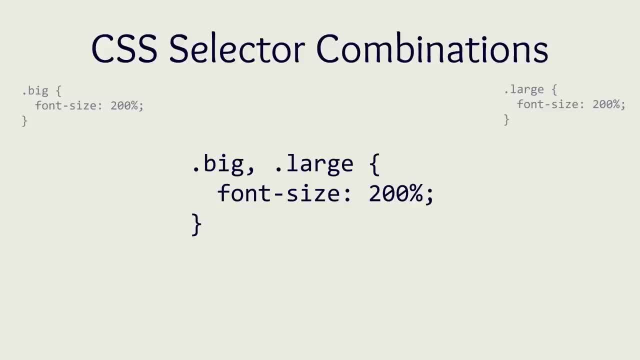 can be used together to create even more complex combinations if needed. There is also one other form of selector, the everything selector, that is used to select every element on the entire webpage. This selector is defined as the asterisk symbol and is only really used to set some defaults for your entire webpage, such as font family. 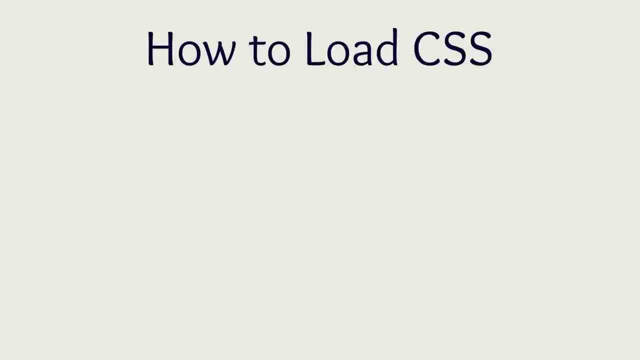 The last thing we need to discuss before writing some CSS is how to load the styles we write into our HTML page. There are three main ways to do this. The first, and by far worst, is to use inline styles. An inline style is CSS that is written directly inside an HTML element. 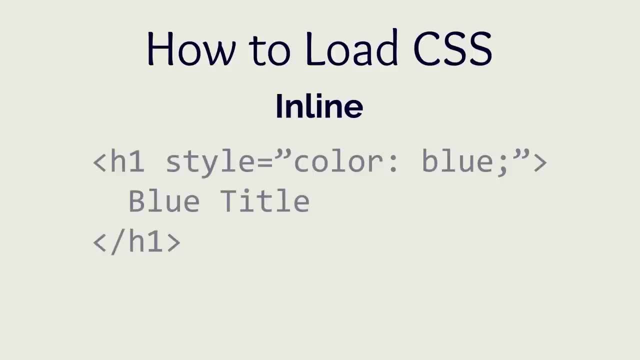 and thus does not need a selector. This is done through the use of the style attribute. This is a terrible idea, though, since HTML is meant for the content only, and mixing CSS styles into your HTML elements adds presentation to your HTML, which is meant for CSS files. 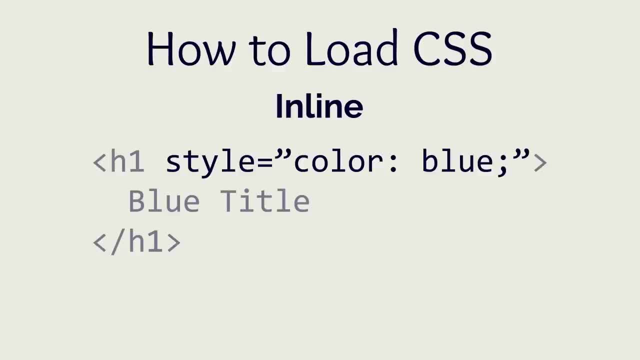 It prevents us from reusing those styles anywhere else, since they are written into the actual HTML element. Lastly, depending on the styles you use in inline, your page may load slower. The second option of using the style HTML element is slightly better, but still a bad idea. 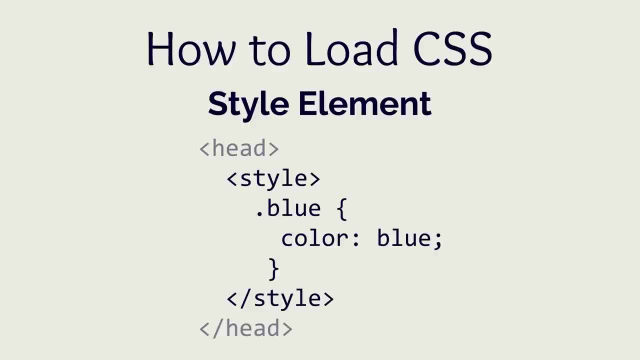 The style element is an HTML element defined in the head and formatted exactly like a CSS file. The problem with using the style element, though, is that the presentation of the webpage is defined in the HTML file and not a CSS file. The styles you define in the style element. 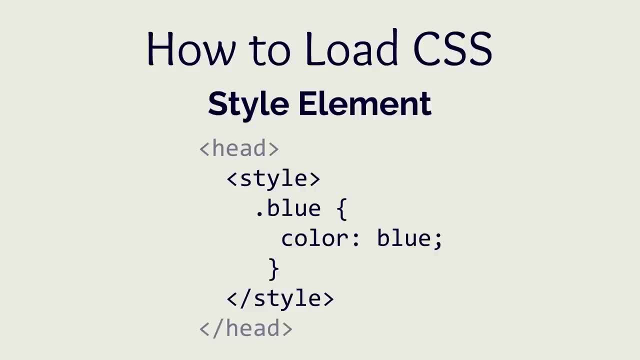 are also only available on the page you define them and are thus not reusable. The final and best way to define CSS styles is to use a separate CSS file and link to it from the HTML. All of the styles for the entire webpage can be defined in one or more CSS files. 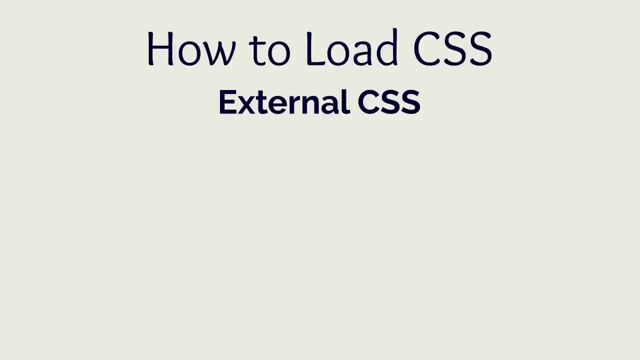 and they can be added to any webpage by using a simple link element inside the head. The link element is a simple element that can be used to link files to the HTML, and its main use is to link CSS files. The link element is also an empty element. 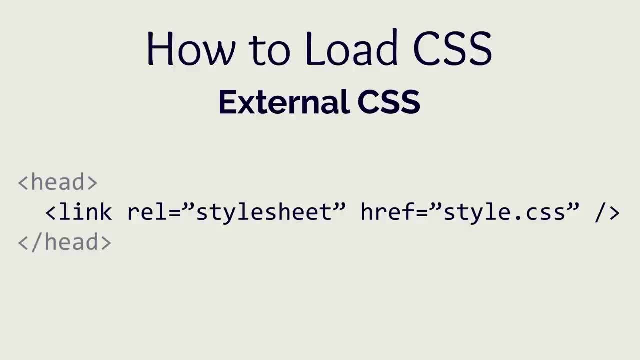 that uses the rel attribute, which stands for the link element. The link element is also an empty element that uses the rel attribute, which stands for relationship, to define the relationship between the linked file and the HTML document. In the case of CSS, the rel attribute will be stylesheet. 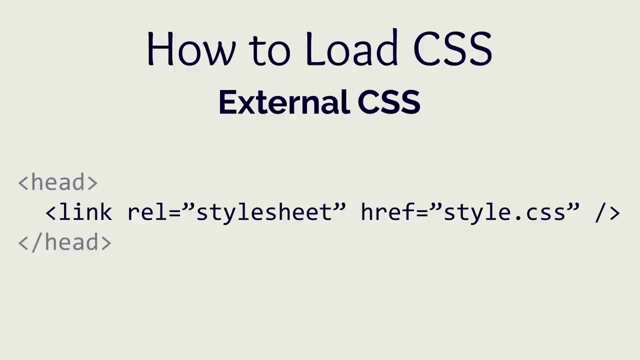 since CSS is a stylesheet for the HTML, The only other attribute that we need to define is the href attribute. The href attribute works exactly the same as the href attribute of an anchor tag and should point to either your CSS file or the URL of another person's CSS file. 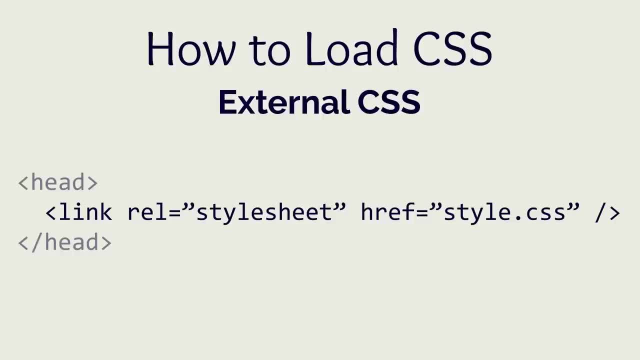 Using external CSS files like this is the best way to use CSS, because it separates the presentation and contents of websites and allows reusability of styles across the website. Now that we have an understanding of how to write CSS styles and select specific HTML elements, 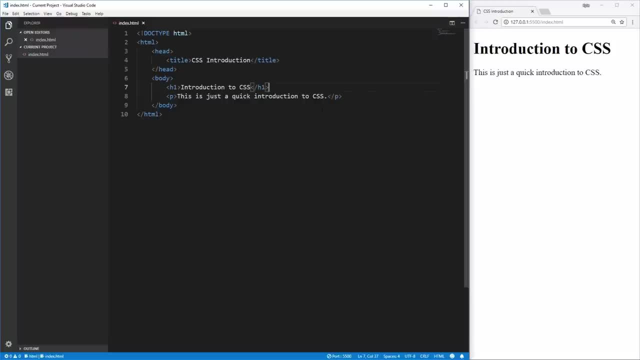 let's jump into a live example of these concepts. As you can see, on the left I have a sample HTML page opened up inside of Visual Studio Code and on the right I have this page opened up in Google Chrome using Live Server To get started. 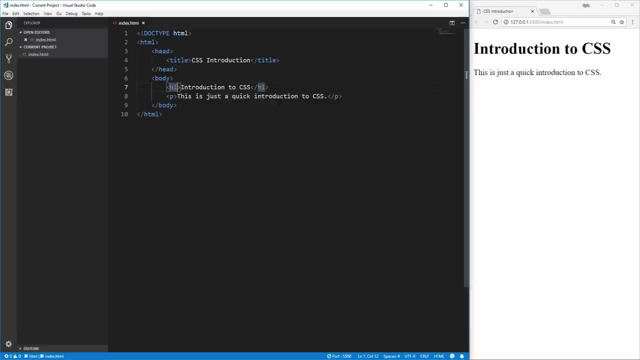 let's use an inline style on this H1 element to turn the text a different color. So we'd use a style attribute here and we would set the color value, since the color property is used to change text color, and we'll set it to a color of red, for example. 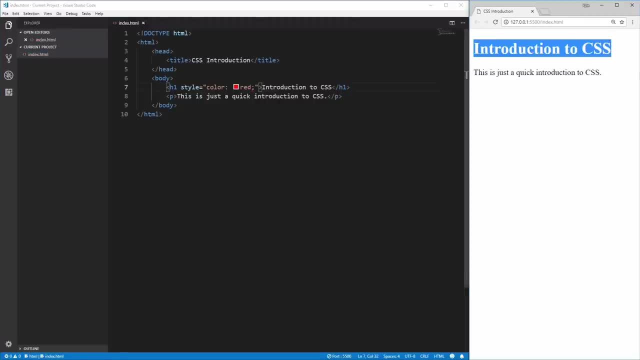 If we save that, as you can see, our text will change to red. But, as we know, using these style attributes is a bad idea. Instead, let's use the style tag inside of the head and use the H1 selector to select the H1 element. 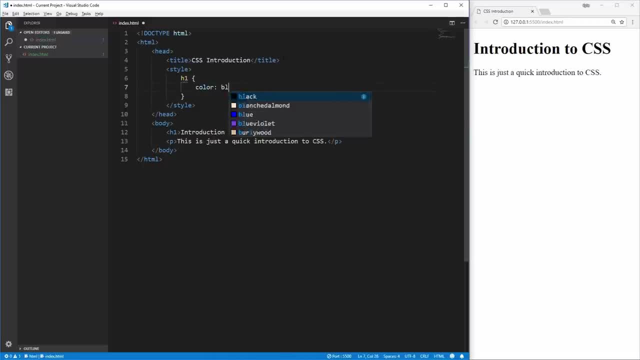 and we'll all set the color to blue this time. Save that and we can see the color is blue. But again, we know that this is not the most optimal way to do it. Instead, let's create a new file called stylescss. 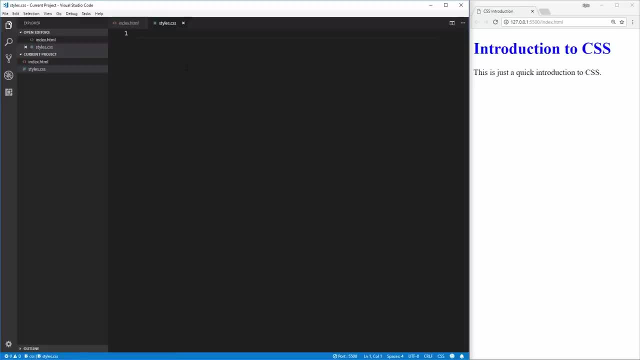 Inside this stylescss file, let's put our H1 selector and set the color to green. Now, in order to get this style to load in our page, we need to use a link tag here, which the rel- is going to be stylesheet, and the href. 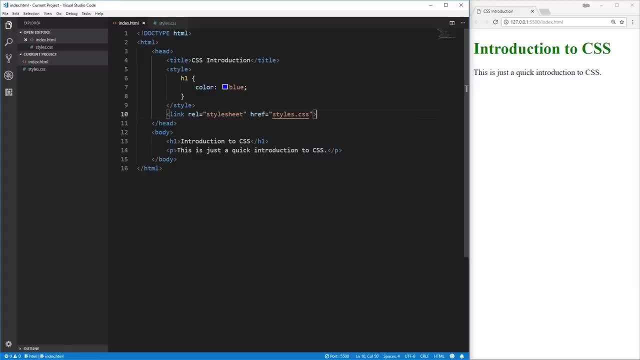 is going to point to that stylescss file. Now, if we save that, you can see that our text changes to green. If we were to move this link tag above our style tag, for example, you see that our text is still blue. 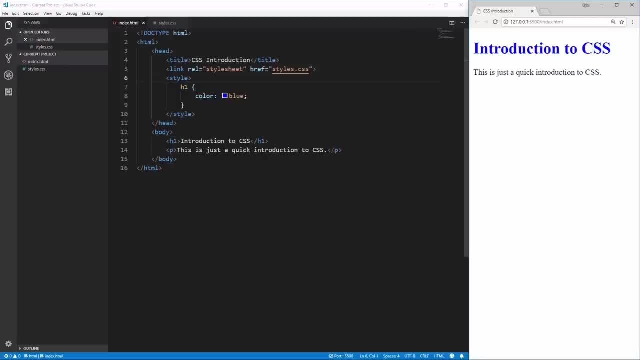 This is because CSS takes whatever the last defined style is for an element, So in this case, the H1 setting the color to blue is below the import of this link, so our text is blue. If we remove this style, though, you'll see that when we save it. 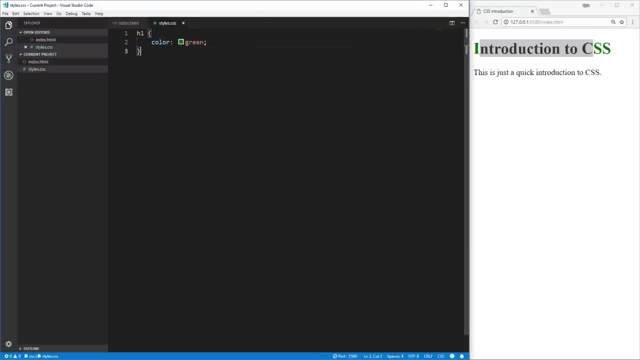 our text turns back to green because it's loading this style in here. We can show that example again by putting the H1 here with a color of red. this time and now, when we save that, this text will change to red because this selector is after this selector. 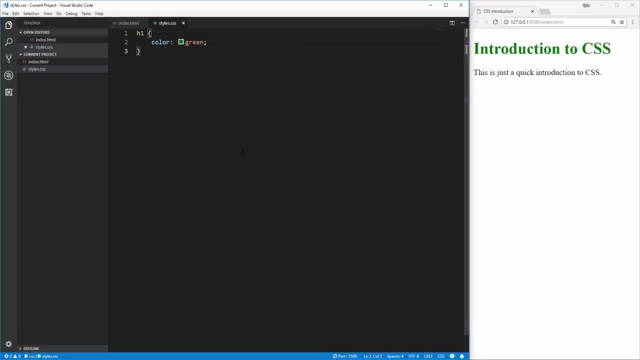 Now that we've finished importing all of our styles, let's dive a little bit more into how the styles are actually applied. To do this, let's add a class to this H1 and we'll give it a class of blue And instead of our stylescss. 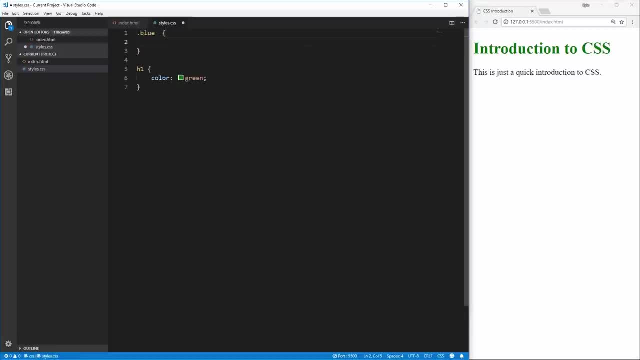 let's add that blue class selector in here and give it a property and value for color to be blue. Now when we save it, we see that our color changes to blue. but you would think that the color would be green, since this H1 selector comes after the blue class selector. 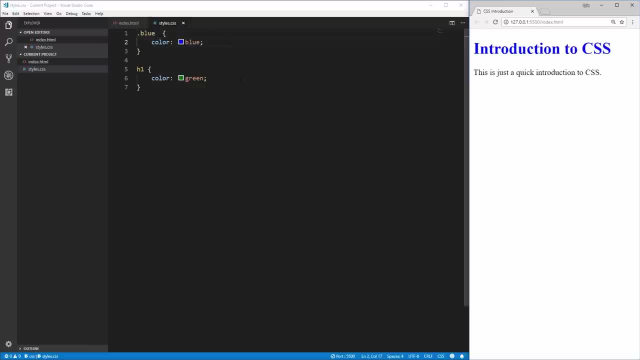 but CSS actually puts different values onto these different selectors. Element selectors are the lowest level selector, which means that they're always overridden by other selectors, such as the class selector. The class selector is then the next in line and it is overridden only by the ID selector. 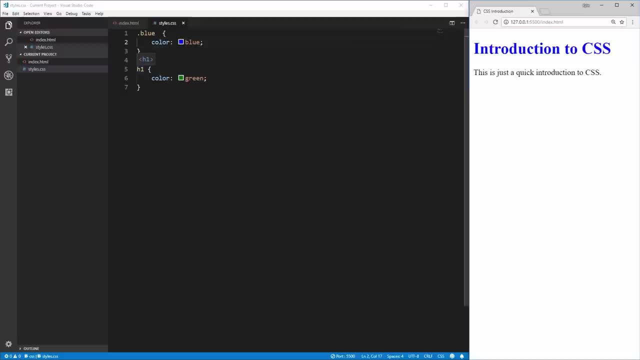 So, in order, the ID selector is the most important, then the class selector and then the element selector. So if we were to look at an example, we have an ID here, class and another class. this selector would have a higher specificity than this selector that had. 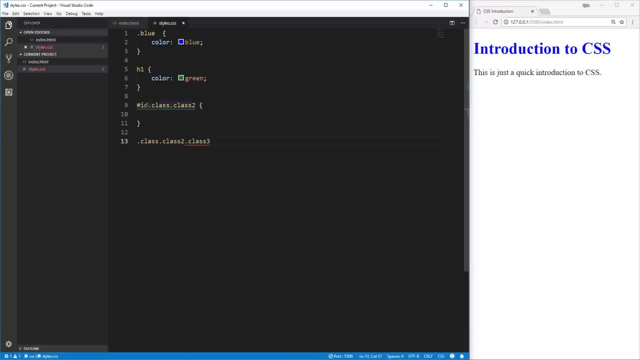 three classes. that is because there is an ID here, so the ID setting has about a value of one. and then we have two classes here, so the class value would have two, but this has three classes and no ID. so since there is one ID on this one, 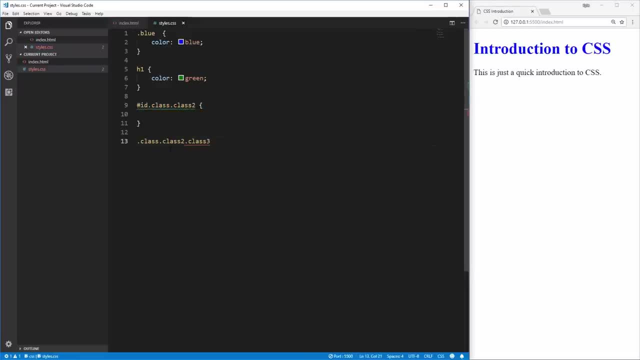 it would be a higher specificity, so anything in here would override anything in here. Essentially, the easiest way to look at this is to first count the number of IDs in the selector. If the number of IDs is equal, then go onto the number of classes in the selector. 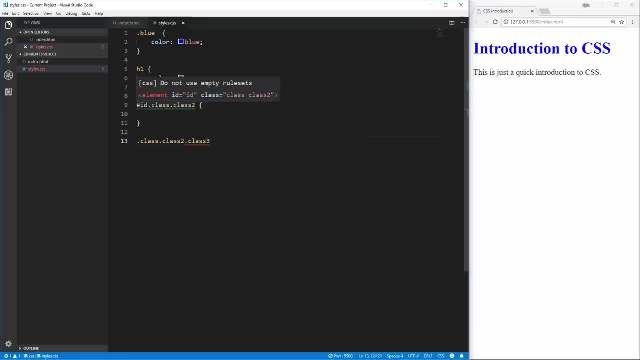 If the number of classes is equal, then finally go onto the number of elements in the selector. If that is also equal, then whichever one is defined last is going to be the one that is applied In any case, if the ID number, class number or element number 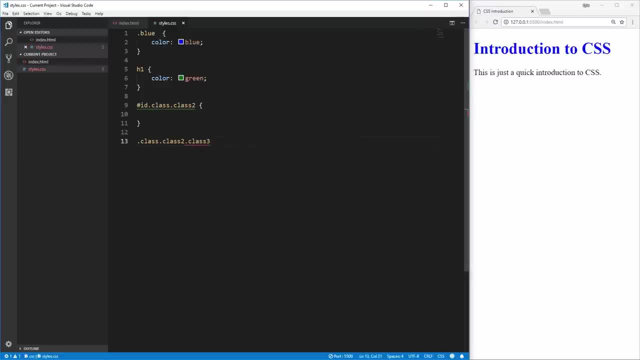 is greater. when you get to that step of adding, that is the style that will be applied, Also if we have an inline style. so, for example, in here, if we put style and we set the color to be equal to black, for example, this will override everything. 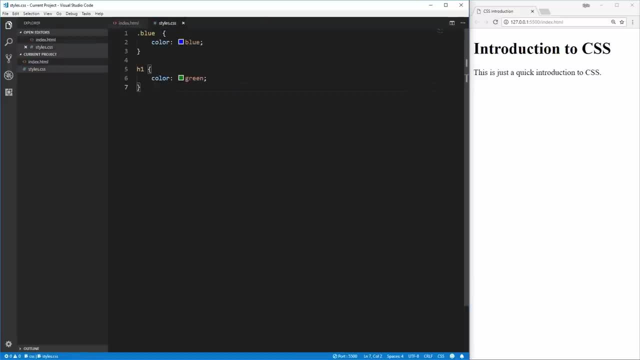 Anything defined inline like this overrides everything in your stylesheet, no matter what. Most HTML elements have a set of default CSS that is applied to them. As you can see, the h1 tag over here has margin on the top and bottom of it and this p tag has this black text. 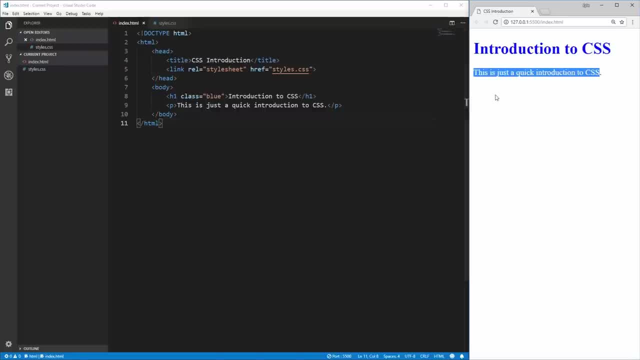 that is because the text color is inherited from, whatever the parent is. This is apparent. if we style the body tag in here and we set the color to be red, This will change all the text in our entire application to be red. that is underneath the body tag. 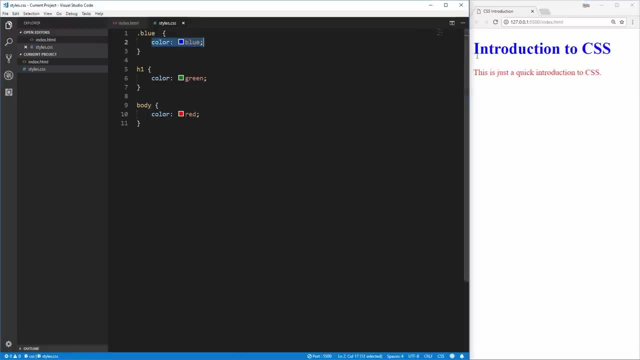 unless otherwise specified, such as this blue selector here that is specifying the h1, should be blue. This is because the default value for text color is inherit, which means it inherits whatever its parent's value is. Since we've been talking about color so much, let's dive into the different ways. 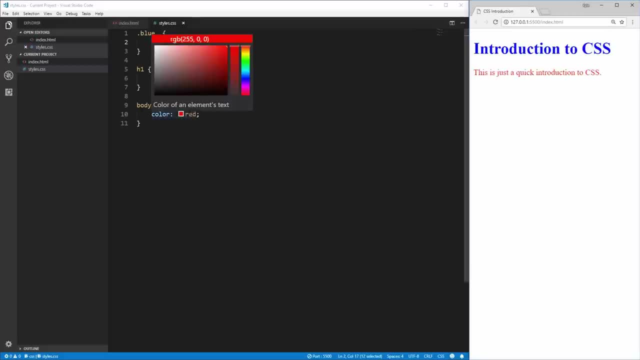 that you can define colors in HTML. By default, you can use these simple color selectors of red, green, blue, pink and various other different colors, but sometimes you want to get more specific than these very generic colors. In order to do that, we'll use 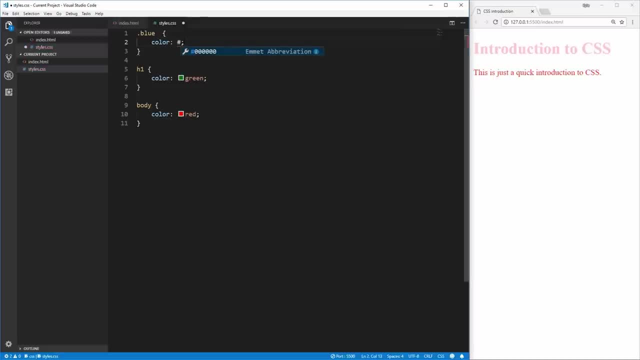 hexadecimal colors in order to set these. A hexadecimal number is similar to our decimal system: that goes from 0 to 9, but hexadecimal goes from 0 to 15.. In order to represent these numbers that are above 9, hexadecimal uses the letters. 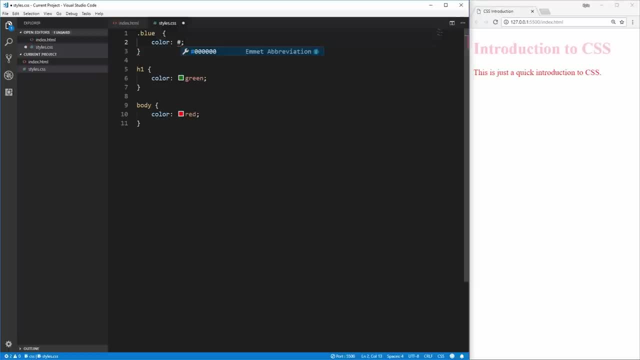 a, b, c, d, e and f. If we wanted to write 15 in hexadecimal, you would write the pound sign, followed by an f, which would be 15.. For using colors, this hexadecimal is broken up into three distinct. 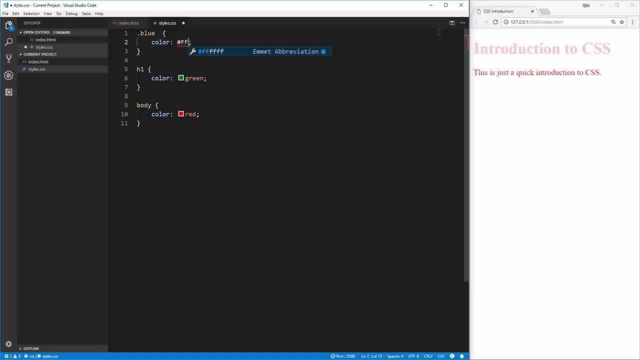 parts of two digits each. We have the first two digits, the second two digits and the third two digits. Each set of these digits represents a different color. The first two digits represent red, the middle two digits represent green and the last two digits. 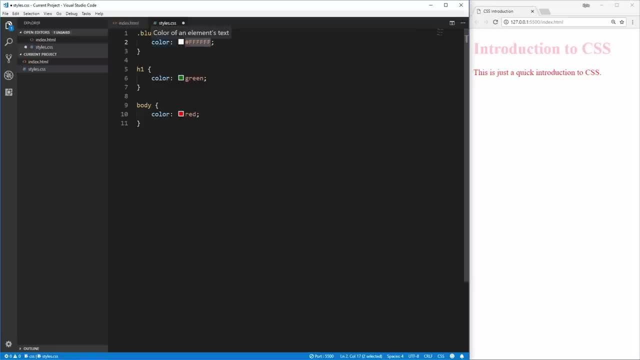 represent blue. This is on a scale from 0 to double f, where double f is equal to 255 in decimal. The smaller the number, the less of that we have. If this was 00,, then that means there is no red at all. 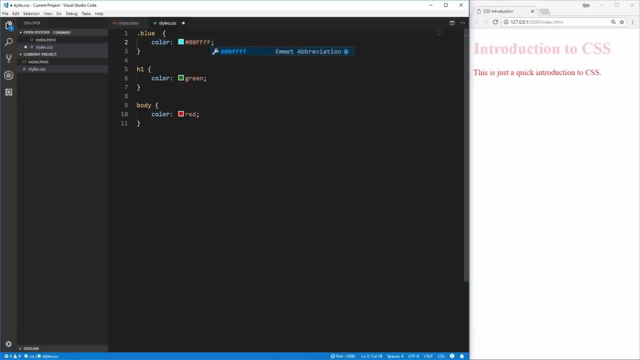 If this one was ff as it is, that means we have all the most amount of blue possible. If it was just blue, we would use 00 for red, 00 for green and then ff for blue. If we save that, we get a blue color. 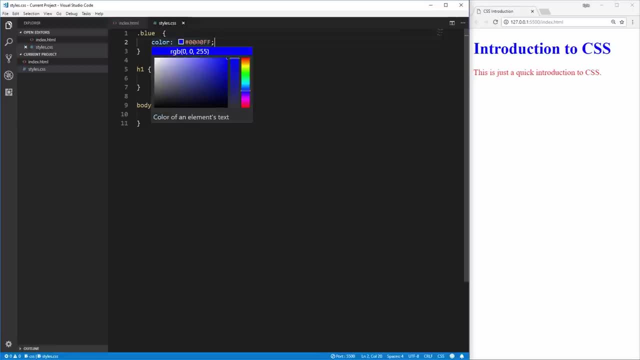 This is a little bit difficult to wrap your header around, so there are other ways to define colors in CSS. One of those ways is using RGB. RGB is just like the hexadecimal version, but it is broken out into three distinct sections. We have red. 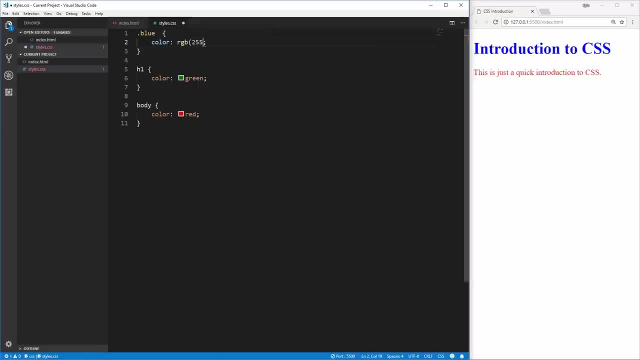 which goes between 0 and 255, and this is in decimal, so we can just write 255 if we want entirely red. The next value is going to be green again, so we can just do 255.. The last one is going to be blue. 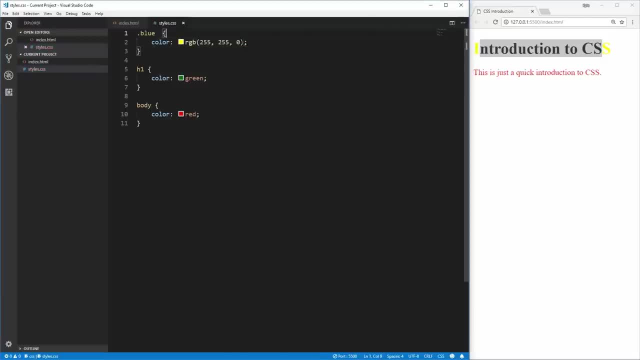 and let's just say that is 0. If we save that, we get yellow. Another way if you wanted to have a partially transparent color is you could use RGBA, where then we have one more value that goes between 0 and 1,. 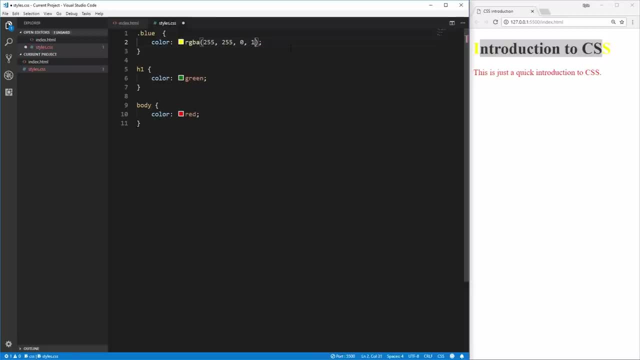 which is going to be the transparency. If it is 1,, it means that it is fully opaque, and if it is 0, then it is going to be entirely transparent. If it is 1,, it means that it is partially transparent. 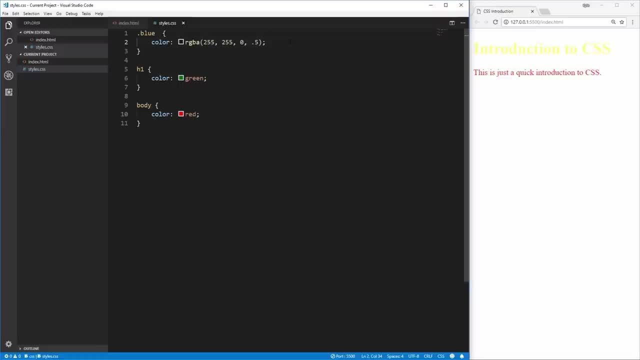 This partial transparency can also be achieved by using the hexadecimal version of the color, and we will just have an extra two digits at the end of the hexadecimal which represent the transparency. So if we wanted to do black, we would do 00,, 00,, 00,. 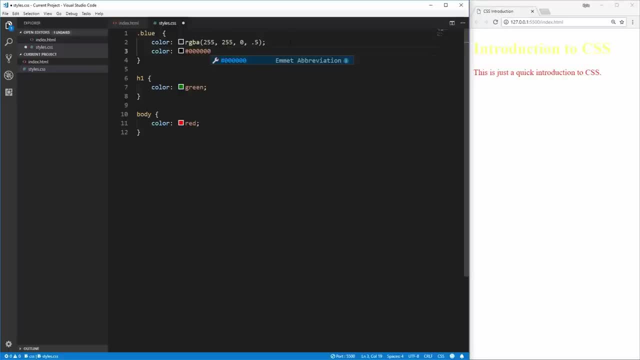 since we have 0 red, 0 green and 0 blue, and then the final value will be the alpha value, which will be between 0 and 255 again. so if we want it to be entirely opaque, we would do FF. 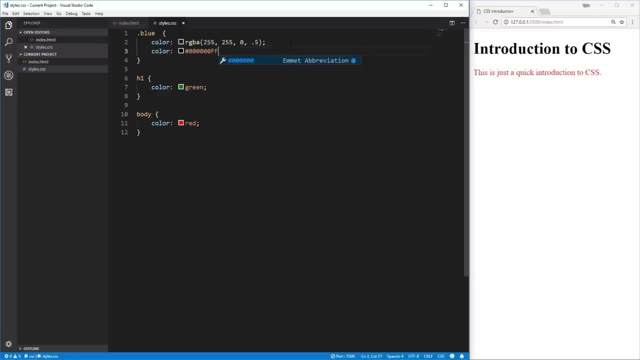 save that and we get entirely opaque black. and if we wanted it to be entirely transparent, just 00, and that will make it entirely transparent. The last way to define colors in HTML is using HSL, which stands for hue saturation. 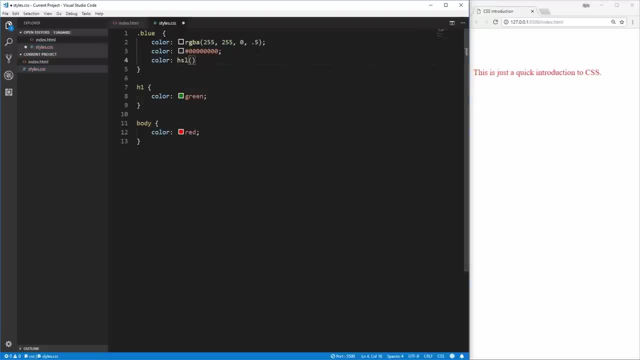 and lightness. The first value, hue, goes between 0 and 360, and determines which color you are going to be using. we will just use 0 in this example. Saturation goes from 0 to 100% and determines how colorful 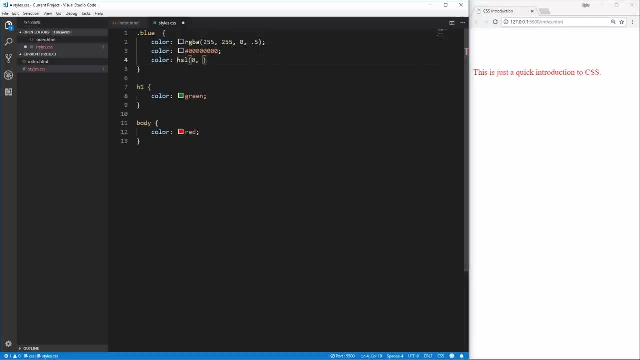 this color is: At 100% saturation, it's as bright as it can be, and at 0% saturation there is no color in it. it is either going to be black, white or somewhere in between there, So let's just use 100% in this example. 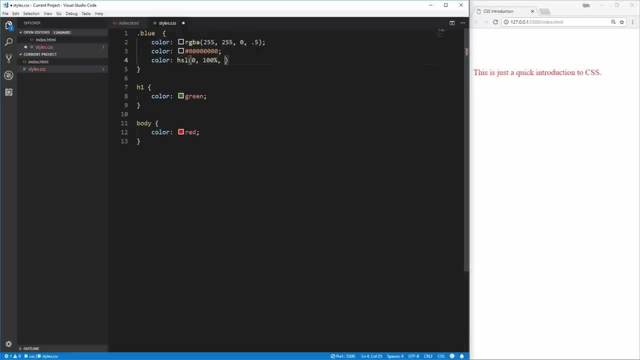 And then, lastly, lightness is going to determine how bright that color is. so at 100% lightness, which is the max, you're going to have an entirely white color, and at 0% lightness, you're going to have an entirely black color. 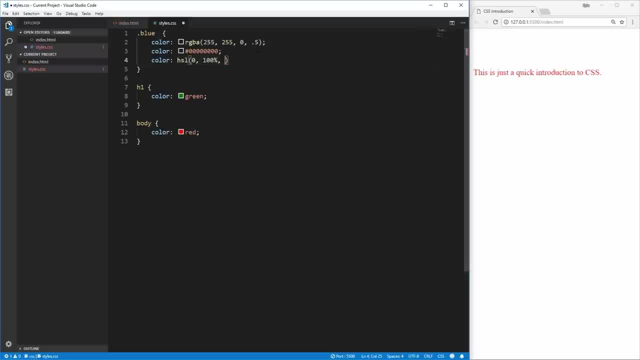 And anywhere in between there is going to be a different shade of that color. So let's just use 50% in this example. If we say that, we see that we get red from this. Also, HSL has an HSLA. 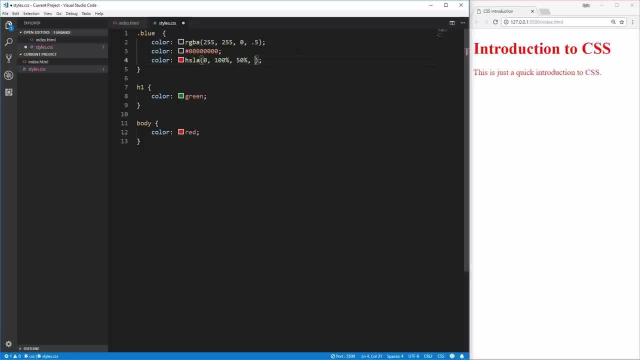 version which lets you put the alpha value or the transparency at the end, where 1 is going to be entirely opaque and 0 is going to be entirely transparent, just like RGBA at the top. Next, we're going to talk about the box model. 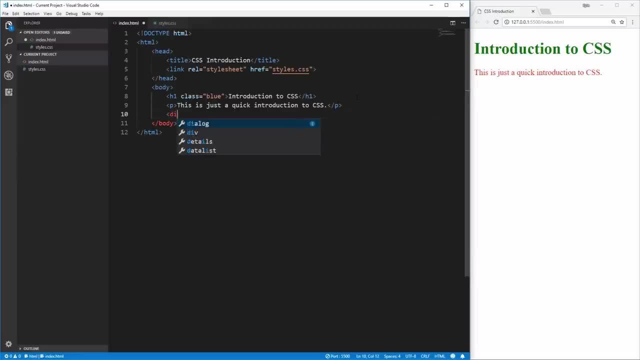 In order to demonstrate this, I'm going to create a new div element and I'm going to give it a class of box. there we go and in the style, we'll style that box element and we'll give it a height and a width. 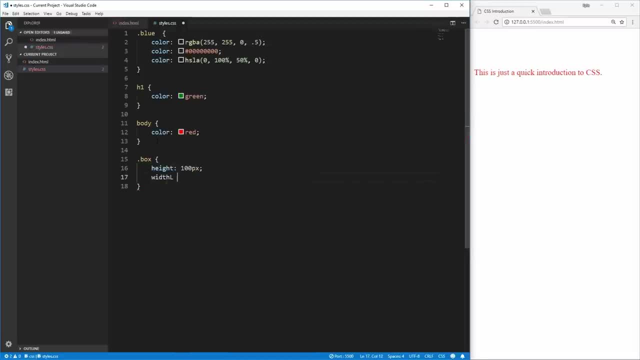 of 100 pixels, a padding of 20 pixels, a margin of 50 pixels and a border that is going to be 10 pixels, and it'll be black. Don't worry about the syntax here. this is really just to demonstrate how the box 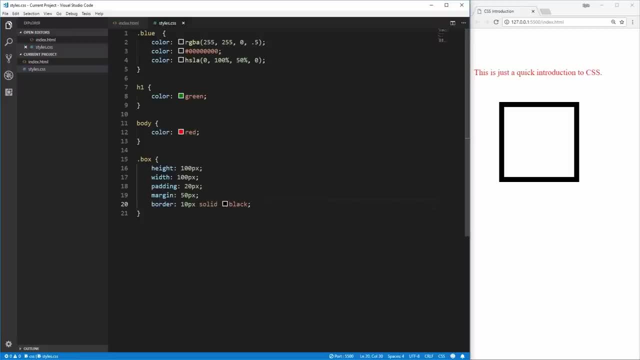 model works If we save that. oh, first let's give it a background background color of red, And now, as you can see over here, we have this red background, we have our black border, but where is this margin and padding coming from? 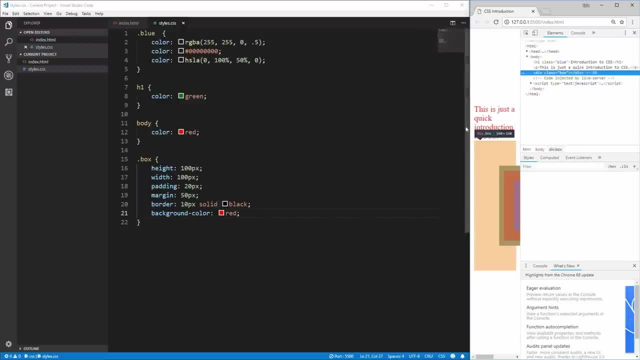 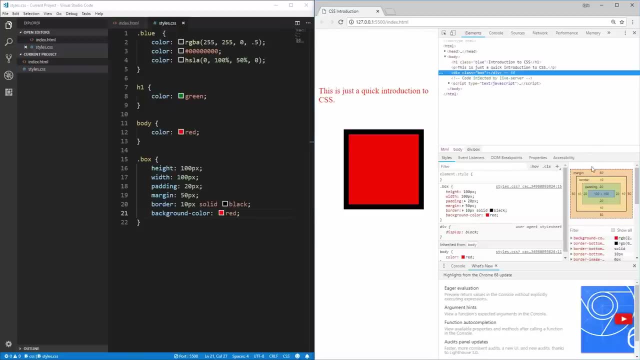 In order to see this, let's inspect this element in Google Chrome, pull this over so that we can actually see, and down here we have the box model. So we have our 100, width by 100 height, which is the actual content of our thing. 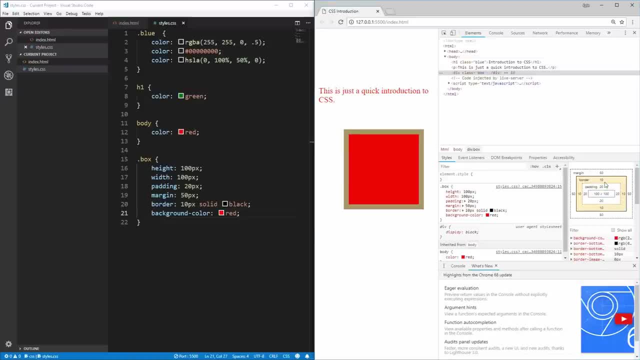 and then around that we have a padding of 20.. And on the left here over here, you can see that it is highlighting. so in blue we have the actual content, 100 by 100,, in orange we have the padding, which is 20 pixels on each. 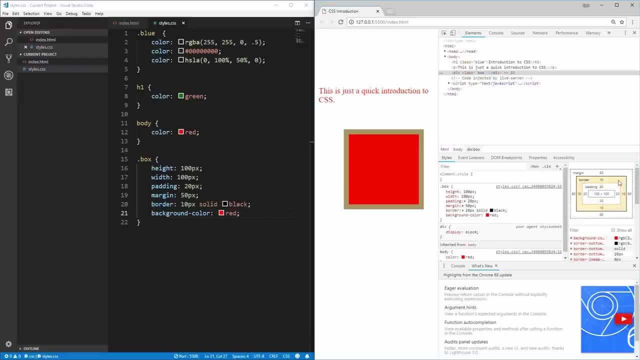 side. next comes our black border, which is 10 pixels around the padding, and then, lastly, our 50 pixels of margin that go around the content. The box model works where the inside of the box model, the very center, is your actual 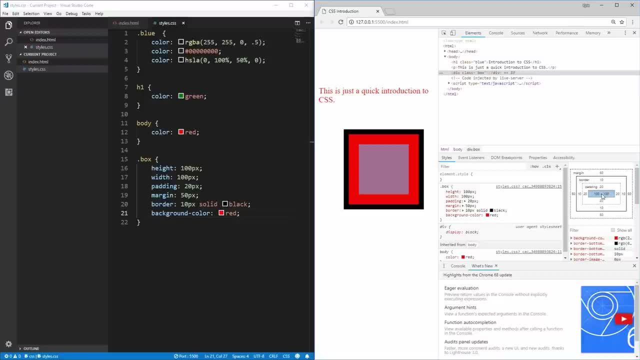 content. This is going to be your text image. whatever it is that takes up that space is going to be there. And then the very next thing is padding. Padding is essentially just spacing between your content and your border. So on a button for 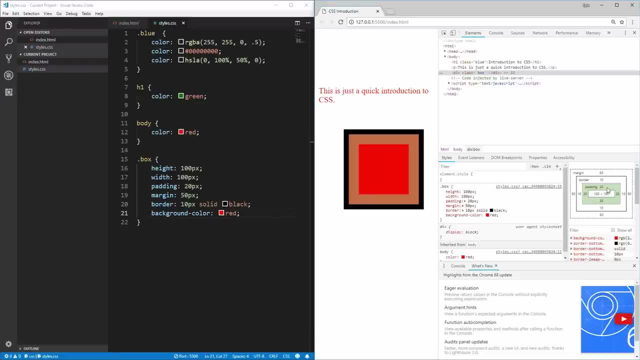 example, this is what allows you to create space between your letters of your button and the actual border around your button, with the background Background also goes on the padding because the background is inside of the border. Then we have the border, which is self-explanatory whatever size you make the. 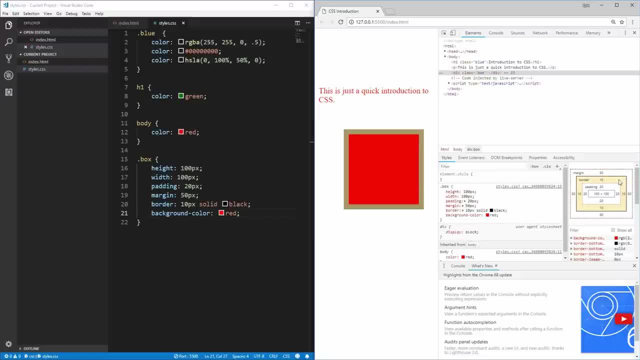 border is how wide the border is going to be. and then, lastly, we have our margin, which is going to be the space on the outside of the border which helps you space elements out from each other. Margin is meant to space. 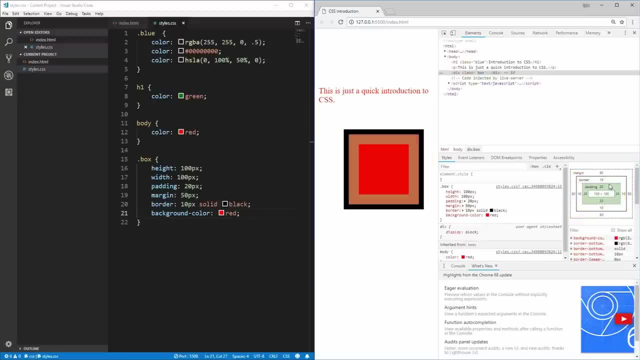 elements around other elements, and padding is meant to space elements around their own border or to add spacing between the element and their actual background. Now that we understand the box model, let's discuss the various different units that we can use on this box model. 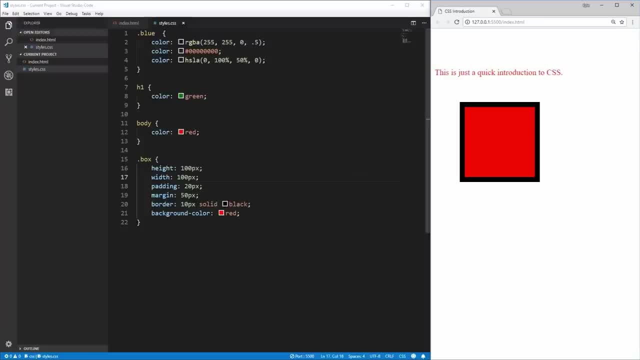 Let's close out of this inspector, widen up our view here and let's talk about, first of all, pixels. Pixels are fairly self-explanatory. they're the unit that you use most of the time when defining content sizes and is going to be a set, fixed width. 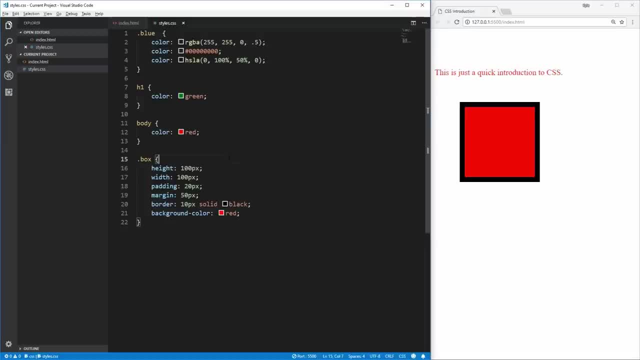 on every size screen. The next unit we have is percentage. Percentage is also fairly self-explanatory and will take up whatever percentage of the given width that the object has inside of its parent. so if we make this width 10%, this box 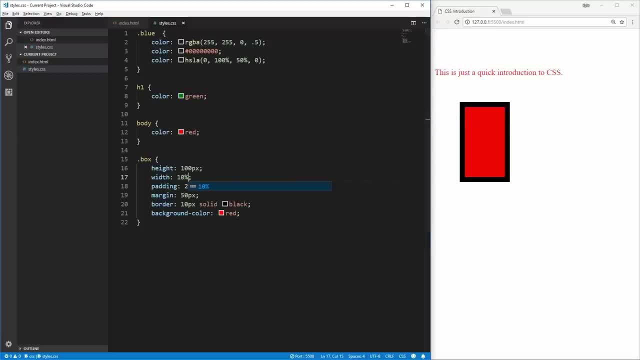 will be 10% of the width of the screen, since the entire width here is how much space we have to work with. The next type of unit that we have is going to be em. Em is mostly used for fonts and font related situations. 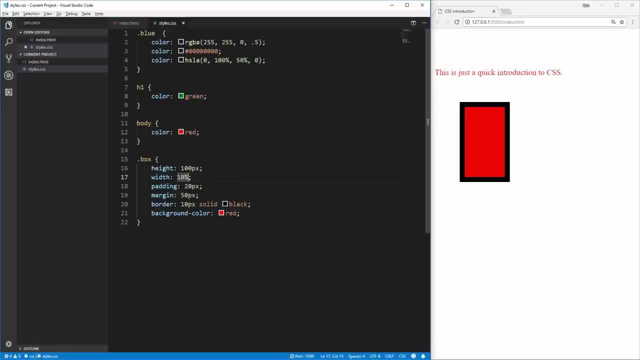 like padding around fonts, and it is going to be. it scales off of the actual font size. So if your font size is 16 pixels, then 1em equals 16 pixels, 2em would be 32 pixels, and so on. 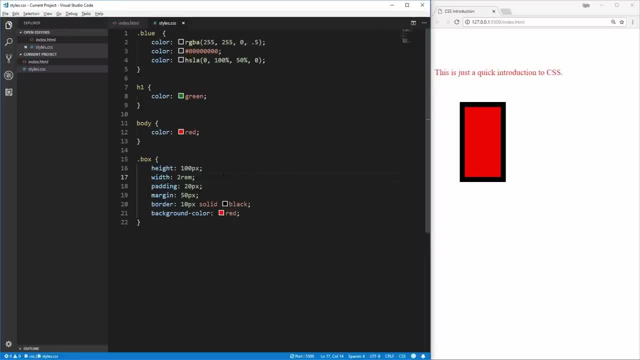 There is also another type of font or scale called rem, which is very similar to em in that it scales off of your font size, but rem scales off the font size of the root of your document. so the very, very base level of our browser. 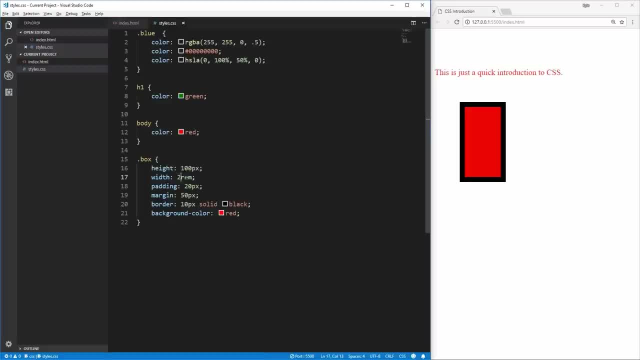 where if we went into the settings and scaled our font size, it would scale off of that, while em scales off of the parent. So this box has a parent of body. so if we change the font size on this body to 20 pixels, you'll see that.